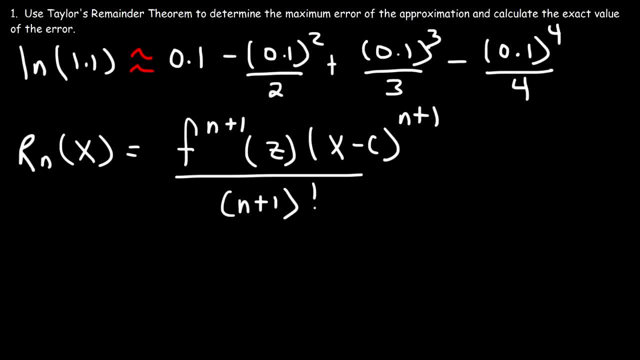 But let's start with n. What do you think n is equal to? What's the value of n? n is basically the last number you see here. n is 4.. Now what about x and c? This number, we're trying to approximate the natural log of 1.1.. 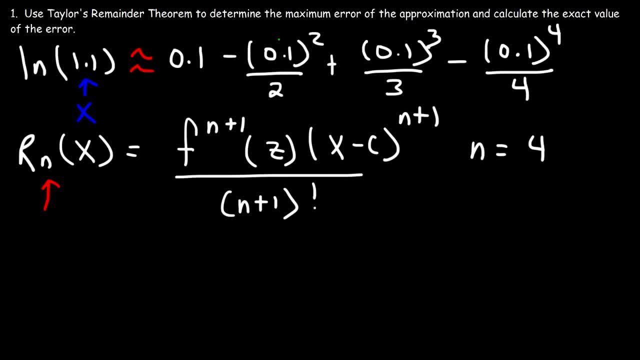 That's your x value. Now the 0.1 that you see in every term, that's equal to x minus c. So if x is 1, I mean if x is 1.1, c has to be 1.. 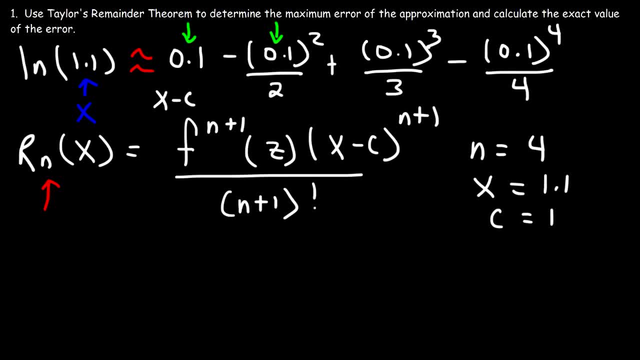 Because 1.1 minus 1 is 0.1.. So we have r4 of x. that's equal to f of n plus 1.. So that's f of 5 of z times x minus c, c is 1.. 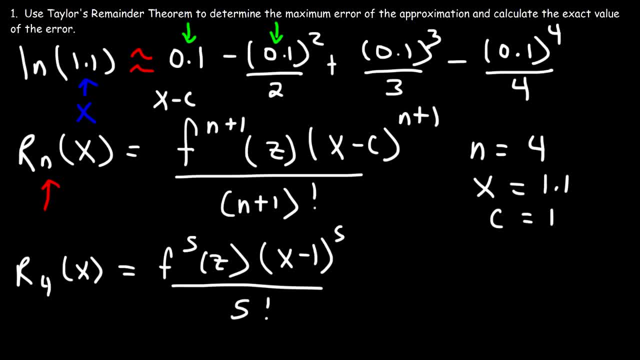 n plus 1 is 5. And then over 5 factorial. Now what is z? z is a number between x and c. So x, we said it's 1.1.. c is 1.. So z could be 1.. 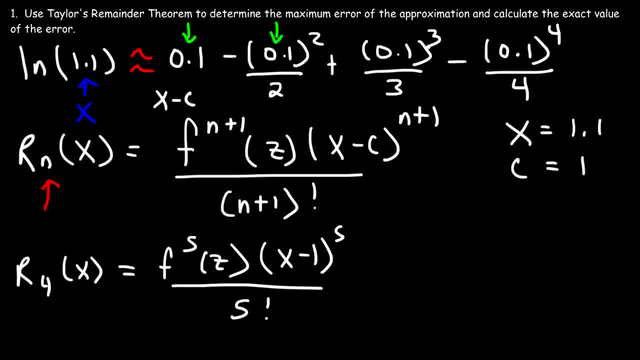 It could be 1.1.. It could be 1.6.. It could be 0.5.. z is a number such that the fifth derivative will have a maximum value. So we need to find what the fifth derivative is. So let's start with the original function f of x, which is the natural log of x. 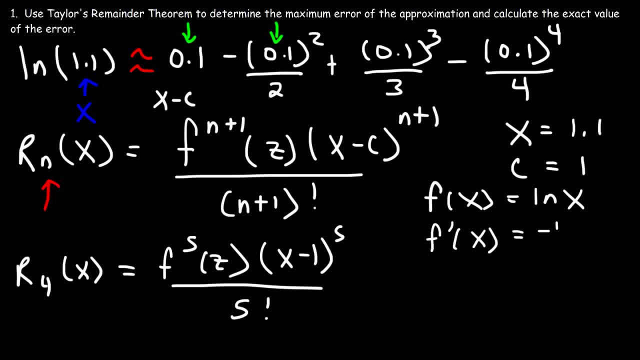 The first derivative is going to be 1 over x, And then the second derivative, 1 over x, is the same as x to the minus 1.. So using the power rule, that's going to be negative 1, x to the minus 2.. 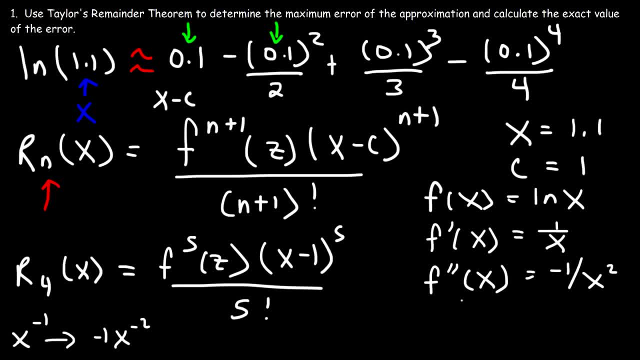 So we can rewrite that as negative 1 over x squared, And then if we take the third derivative, that's going to be 2x to the minus 3.. And then if we take the fourth derivative, negative 6x to the negative 4.. 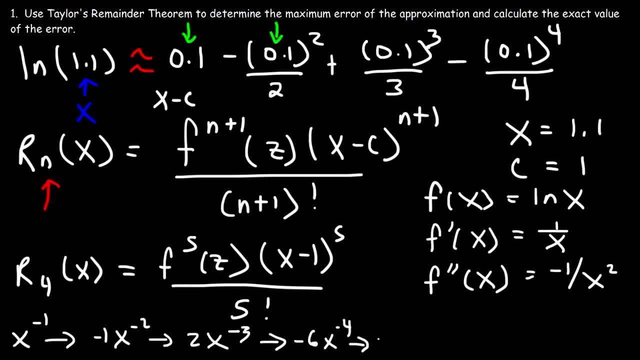 And then the fifth derivative is going to be 24x to the negative 5.. So now that we have the fifth derivative, we have it as 24 over x to the 5th power. Is z going to be 1,, 1.1, or some number in between? 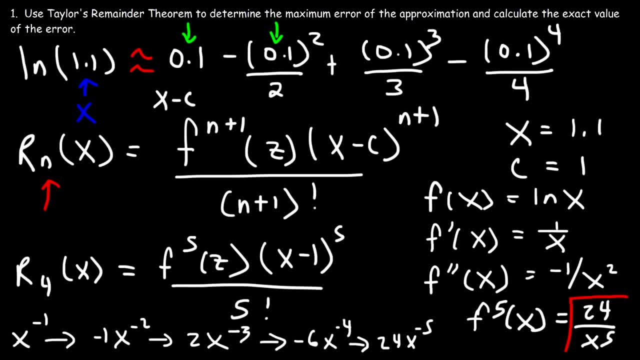 Which of those values will give us the maximum value for the fifth derivative? Notice that x is in the denominator of the fraction And as you decrease the denominator of the fraction, the value of the entire fraction goes up. So we want the lowest x value. 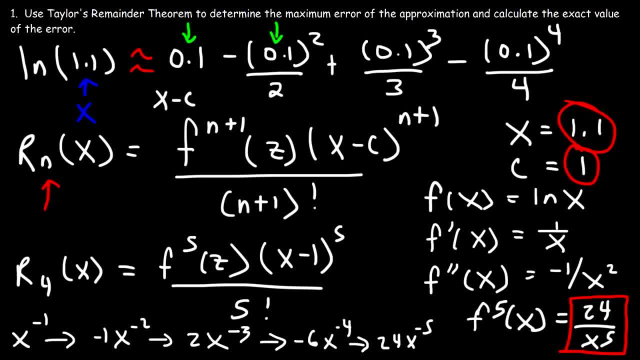 So 1 is lower than 1.1.. So we're going to choose a z value of 1.. So f the fifth derivative of 1, that's going to be 24 over 1 to the 5th power. 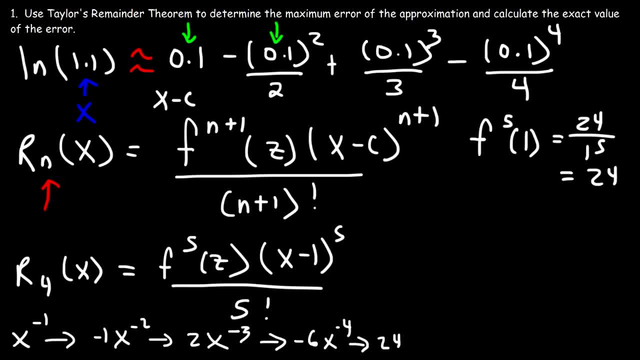 So that equals 24.. So that's r4 of 1.1.. That's going to be: this is 24.. And then plugging in 1.1 into x, that's going to be 1.1 minus 1.. 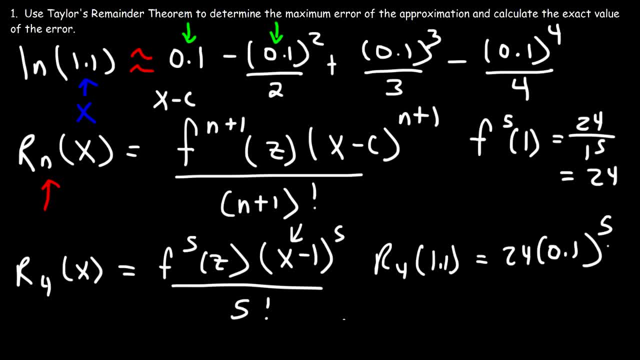 So simply 0.1 to the 5th power And then divide it by 5 factorial. Go ahead and type that in. So the remainder, the maximum value, is 2 times 10 to the negative 6.. So that is the maximum error for this particular approximation. 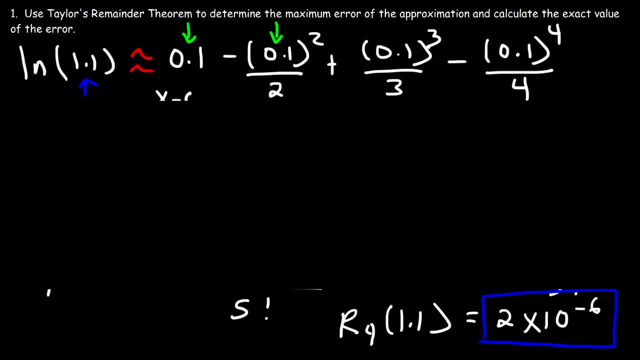 Silence. Now the next thing we need to do is determine the exact value of the error. So we need to find the difference between the natural log of 1.1. And the value of the, the exhaustion there, And therefore the differential value. 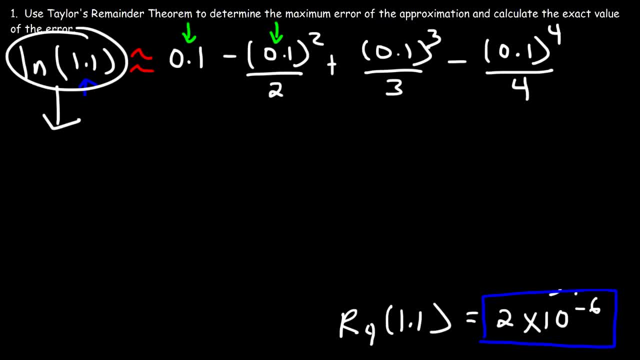 the fourth-degree polynomial at 1.1.. So ln 1.1, that's 0.0953101798.. Now let's evaluate the fourth-degree polynomial when x is 1.1.. So if you type in 0.1. 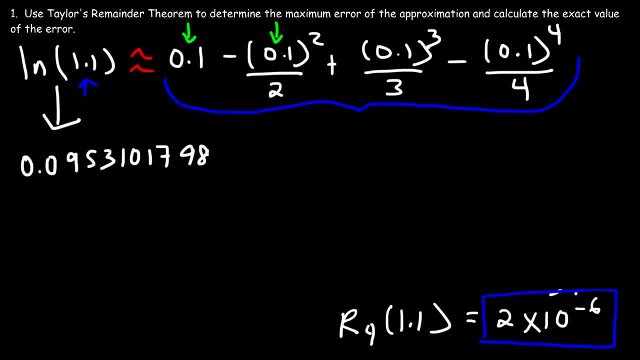 minus 0.1 squared divided by 2 plus 0.1 cubed divided by 3 minus 0.1 to the fourth power, divided by 4, that's going to give you 0.0953083333.. Now, if you take the difference between these two values, 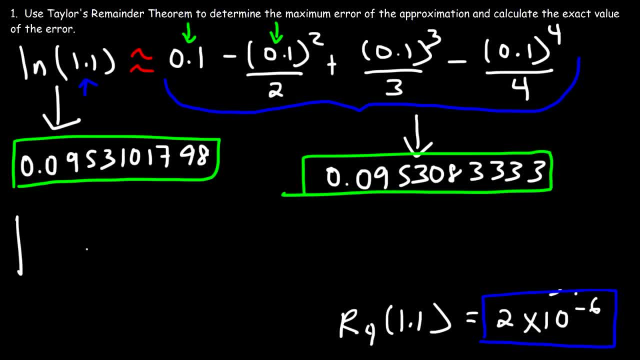 so let's say the absolute value difference between ln 1.1 and the fourth-degree polynomial evaluate at 1.1, that's going to give us the exact error, And so you should get 1.846 times 10 to negative 6.. 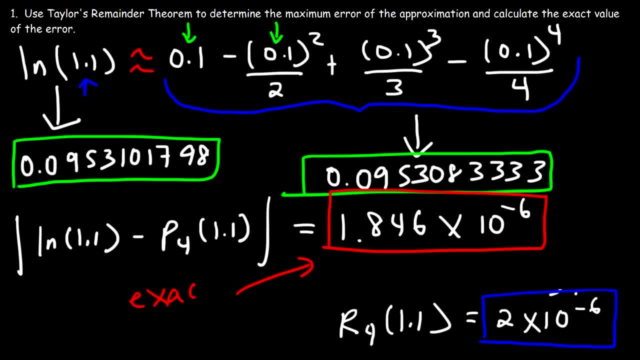 So this is the exact error and this is the maximum error for this particular approximation. So we should expect a higher value for the maximum error compared to the exact error which we do have. Now let's go ahead and work on another similar problem. 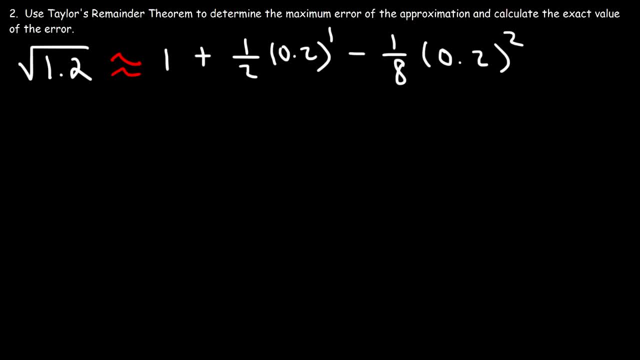 So determine the maximum error of the approximation and also calculate the exact value of the error. So what do we notice in this problem? Well, let's write the formula. to begin with, We know that the remainder, which is going to be the maximum error, that's going to be f, evaluated at z times x minus c, raised to. 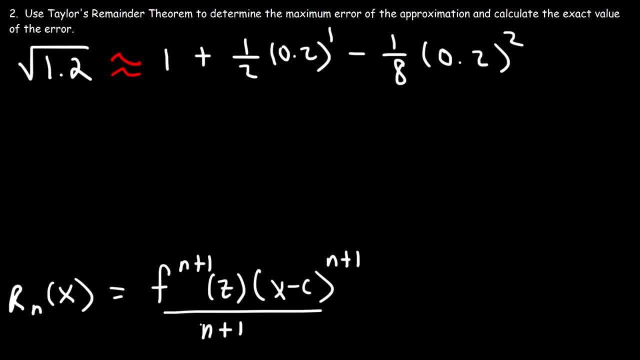 the n plus 1 divided by n plus 1 factorial. So what is n in this problem? Notice that n is 2.. Now, what else do we know? What is x and what is c? X is what we see here, So x is 1.2. now what is the value? 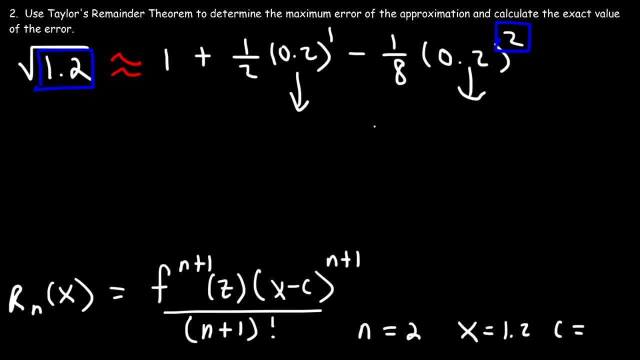 of c. So So notice that the difference between x and c, that's 0.2.. So if you set x minus c equal to 0.2, and replace x with 1.2, then you need to see that c is. 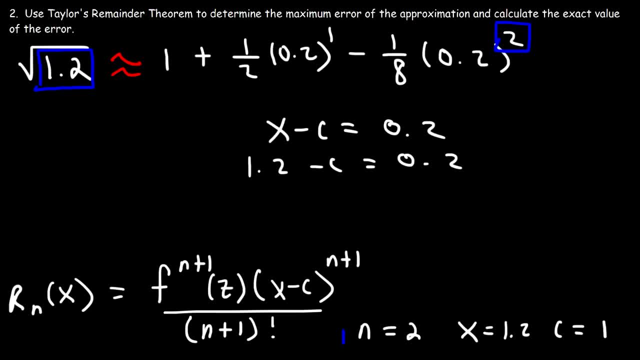 equal to 1.. 1.2 minus 1 is 0.2.. So now we have n, x and c. Now we need to determine the value of z. If n is 2, then n plus 1 is 3, which indicates that we need to find the value of the third. 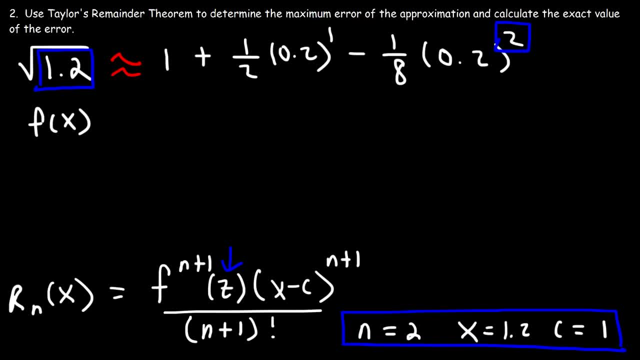 derivative. So what's f? We know that x is 1.2, so if you replace 1.2, we can see that f is the square root of x, which is the same as x to the 1 half. So the first derivative is going to be 1 half x to the negative half. 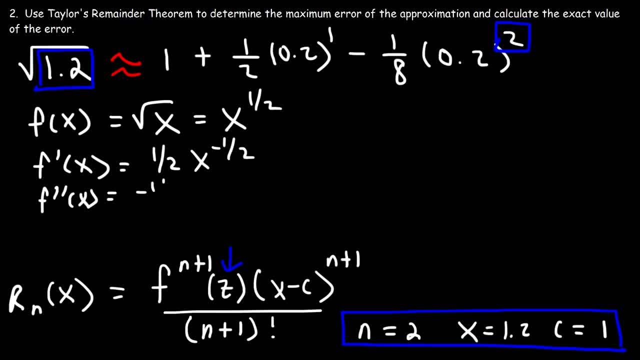 The second derivative. The third derivative is going to be negative 1, fourth, from x to the negative 1, half minus 1, which is negative 3 over 2.. And so the third derivative is going to be negative 1, fourth times negative, 3 over 2.. 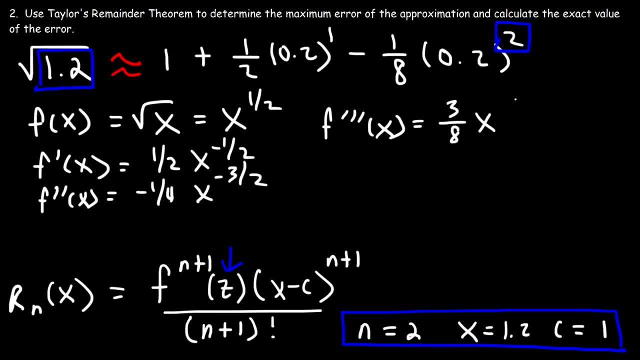 So that's 3 over 8. And negative 3 over 2 times minus 1 is negative 5 over 2.. So I'm going to rewrite the third derivative as 3 over 8, then x to the 5 halves. 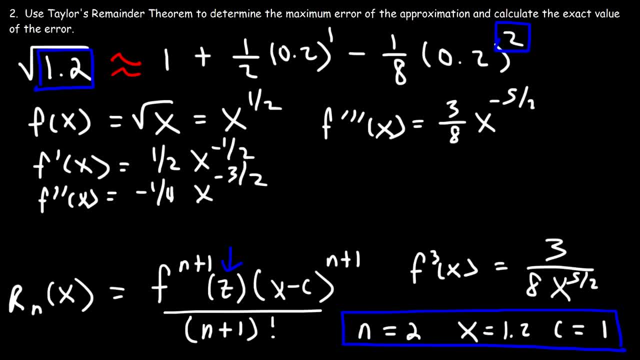 5 halves is 2.2. 0.2., 0.2., 0.25., 0.25. 0.25. and 2.5 is 2 plus 0.5. so we're going to have x squared times x to the 0.5, which. 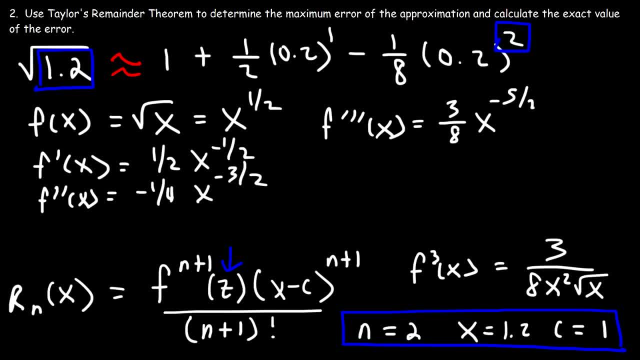 is basically the square root of x, so that's the third derivative. now we know that Z is between X and C, so it's between 1 and 1.2. which one will give us a maximum third derivative value, 1 or 1.2? now remember, if you decrease the 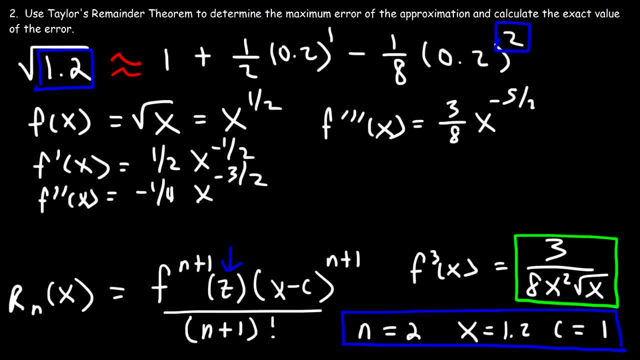 value of the denominator of a fraction, the value, the whole fraction, goes up. so since we're plugging in a number into the bottom, we want to plug in the lowest value, which is C, in this case 1. so we're going to say that Z we're going to set. 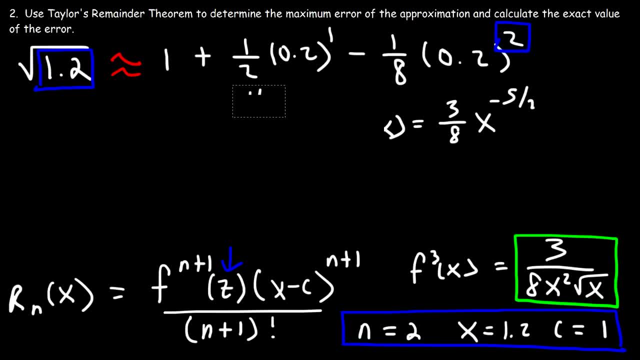 it equal to 1. our goal is to determine the maximum error. so now that we know that Z is equal to 1, we can calculate the error. so n is 2, so we're going to have our sub 2 of X, and that's n plus 1. so this is the third derivative at Z, and then times X, C is 1. 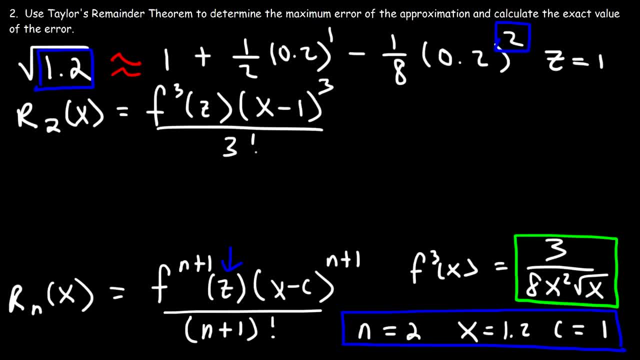 n plus 1 is 3 divided by 3 factorial. so now let's plug in Z and X. so X is 1.2 and this is going to be the third derivative evaluated at 1, and then this is going to be 1.2 minus 1 to the third power over 3 factorial. 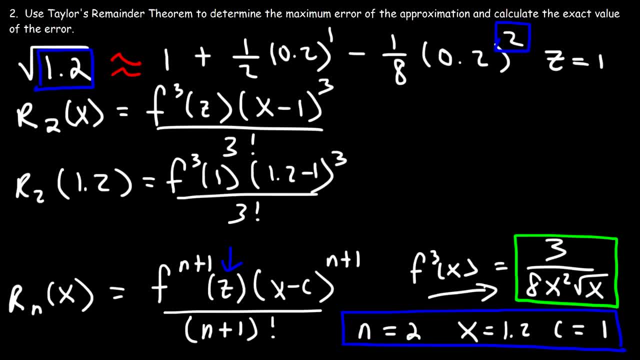 so if we plug in 1 into this expression, it's just going to be 3 over 8. so we have 3 over 8 times 0.2, raised to the third power over 3, factorial. go ahead and type that in so you should get 5 times 10 to the negative 4.